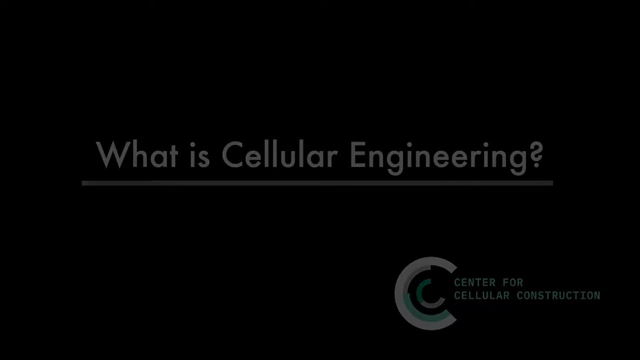 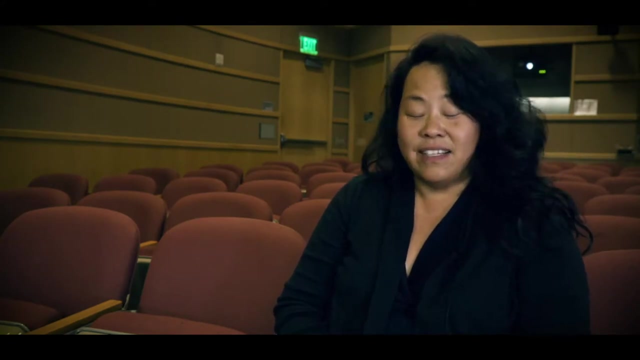 Cellular engineering to me as a biologist is something very different than I thought it would be. As a biologist, I'm really thinking about how cells work, but thinking about how cells work as an engineer is something that I wasn't used to. So during this process of thinking about what 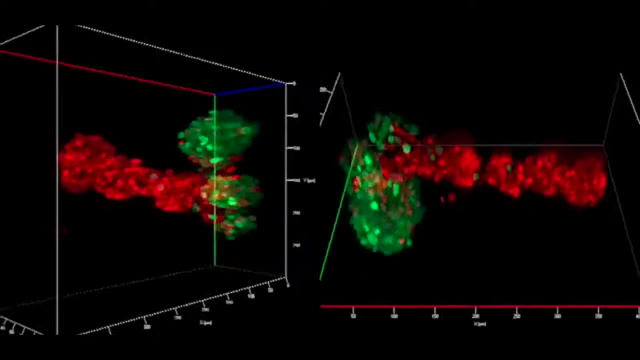 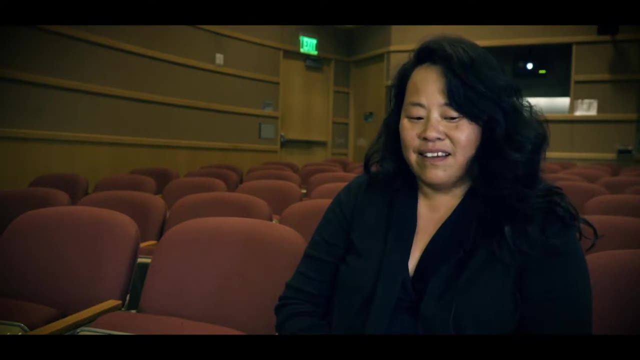 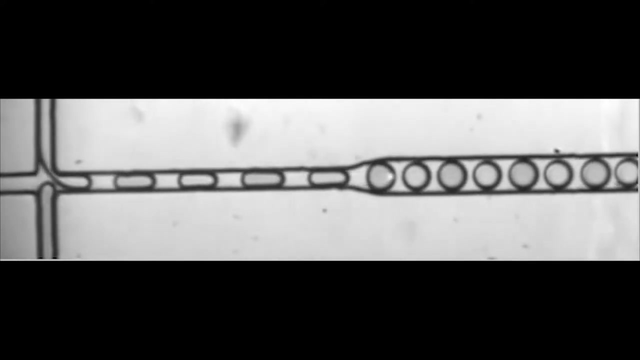 cellular engineering is, has opened my eyes to sort of a different way to look at how cells work and what we can do with cells. So now I think about, not just about proteins and things swimming around in a bag. Now I really think about how, what these kind of properties of those things within 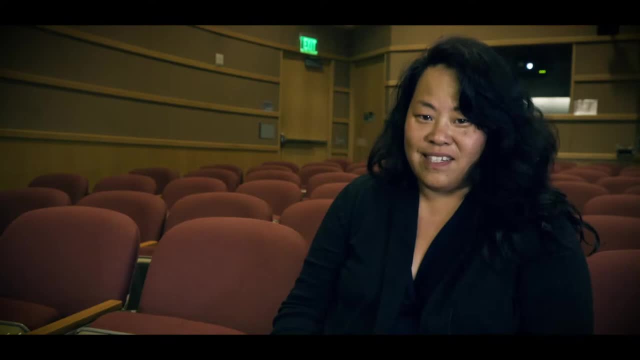 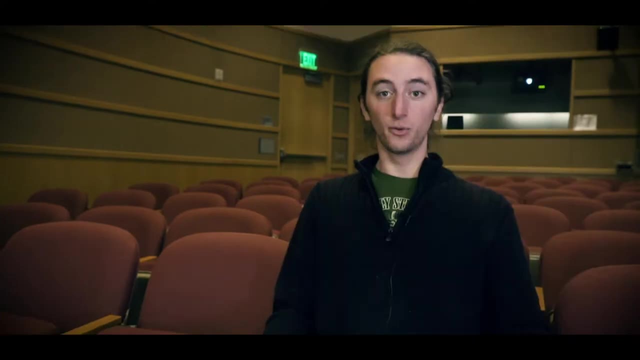 the bags have and how that really determines what a cell does, how big it can get or how small it is or what it can produce. The way I understand cellular engineering is that the cell, it, has a massively complicated structure and has all sorts of different sizes and shapes of organelles. 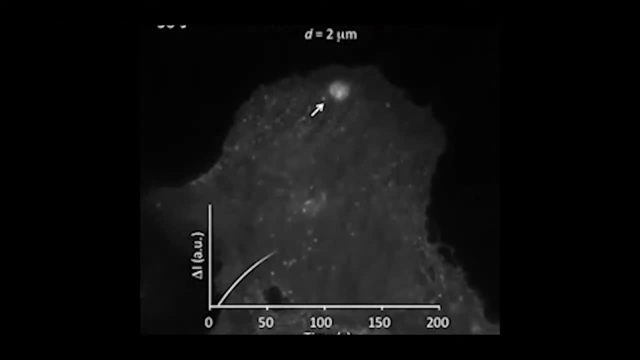 and it's not really clear to us in the scientific community how these organelles are built, because we know that the things that are building them- these, you know, proteins and molecules- are thousands of times smaller than the organelles themselves. So somehow these small structures are. 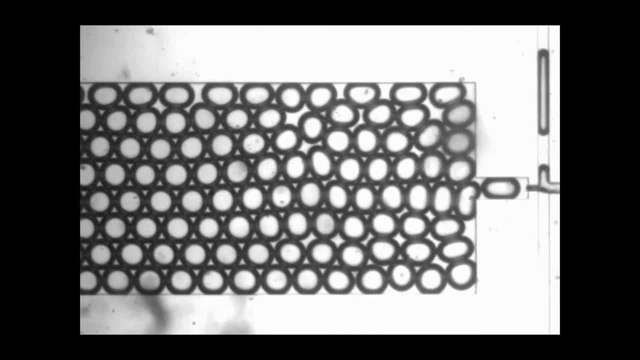 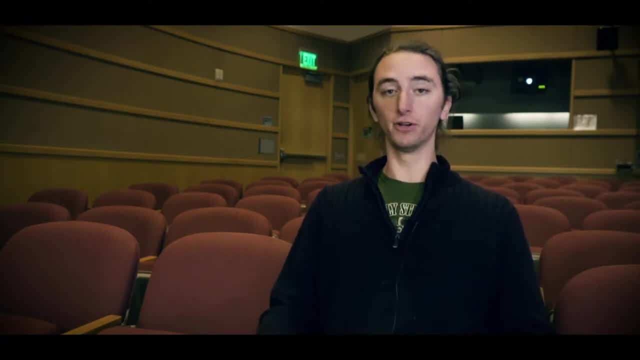 using just local interactions to create these massive structures, and we're starting to know a little bit about different kinds of ways they can do that, but we still don't have a fully complete picture. So I think to me cellular engineering means trying to understand that process better and learning how we can understand it and then, in the future, harness it to create. 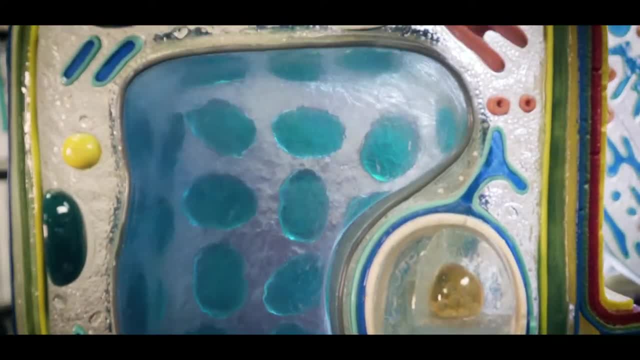 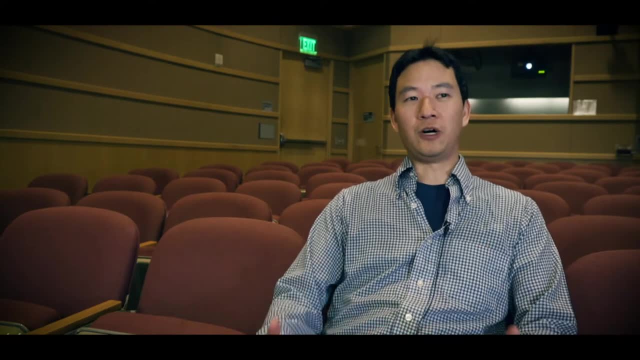 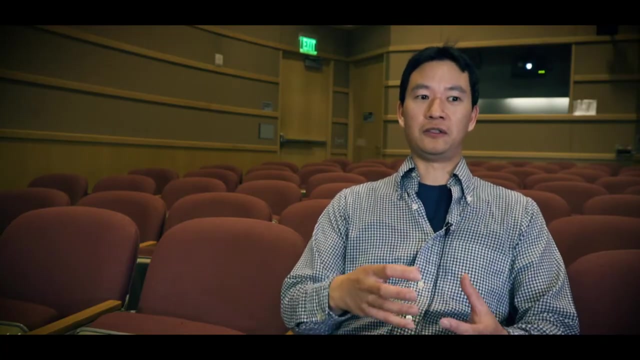 cells that have desired effects, hence cellular engineering. So to me, cellular engineering means being able to design cells with properties that we want, and so that's very kind of abstract. but I think of cells as little structures, little objects that contain objects within them and they 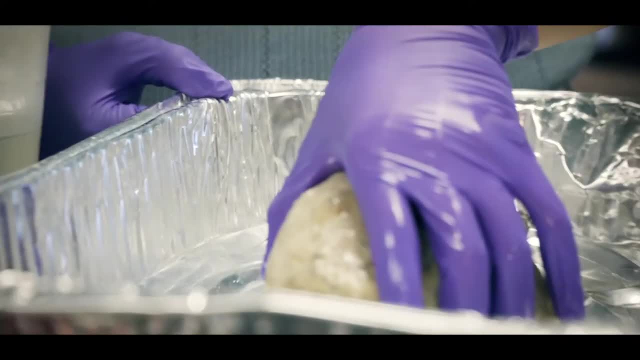 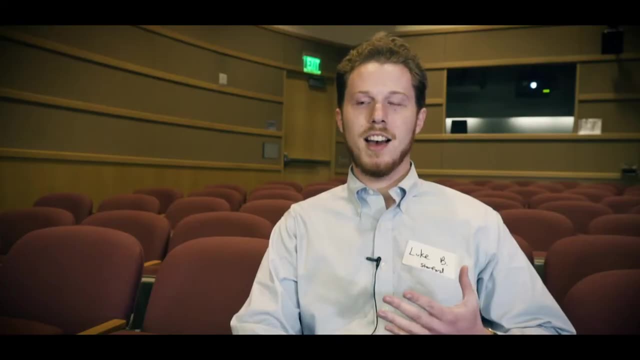 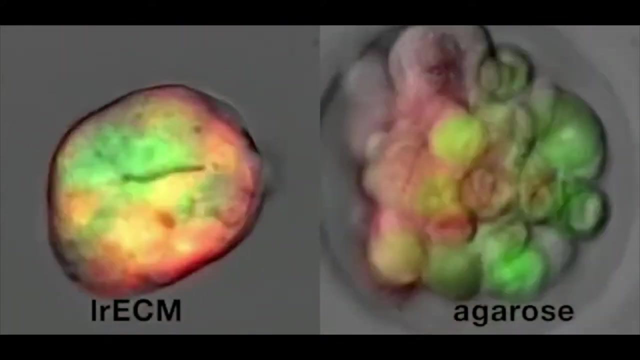 build those objects called organelles within themselves, sort of like we have organs inside our own bodies. A cell is like one of the most complicated chemical systems that we can think of, and what cellular engineering allows us to do is to take advantage of the components of the cell.